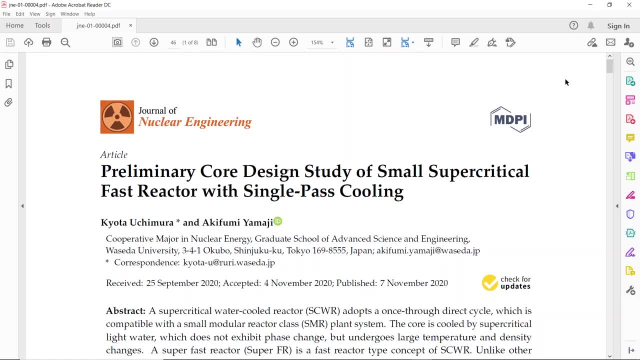 from Waseda University, Japan. The editorial is MDPI. The reason why I choose this publication is because I'm board reviewer of MDPI and of course this is not a top top journal. so it's also interesting to see, because otherwise it will not get a lot of attention. so let's go to see the abstract. 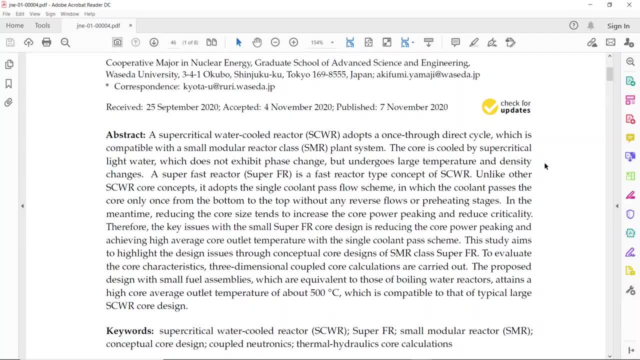 I will read the abstract and then go a bit over it and make some final thoughts. A supercritical water-cooled reactor adopts a once-through direct cycle which is compatible with a small modular reactor class SMR plant system. A supercritical water-cooled reactor adopts a once-through direct cycle which is compatible with a small modular reactor class SMR plant system. 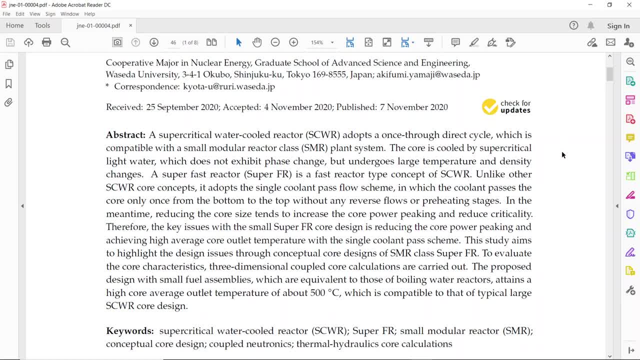 The core is cooled by supercritical light water which does not exhibit phase change, so it means it doesn't boil, but undergoes large temperature and density changes. This is interesting because usually in most of applications you don't consider the density change of water according to temperature, but here, due to the large temperature variation, 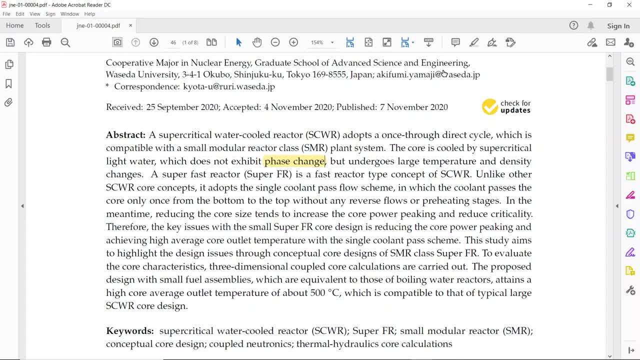 without boiling. it's significant. We'll see later. A superfast reactor is a fast reactor type concept of SCWR. Unlike other SCWR core concepts, it adopts the single coolant pass flow scheme, in which the coolant passes the core only once, from the bottom to the top, without any reverse flow or preheating stages. 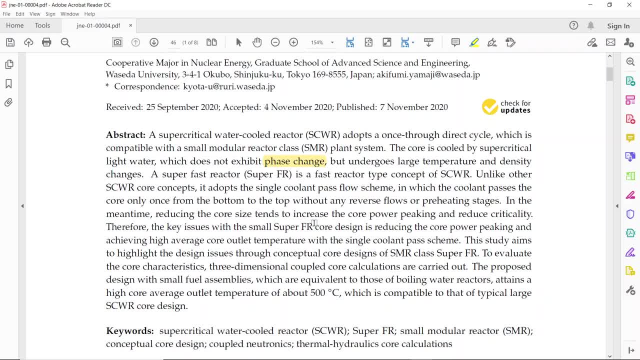 In the meantime, reducing the core size tends to increase the core power picking and reduce the power consumption. I'm not sure about the meaning of this. I guess reduce criticality means reducing reactivity of the whole reactor, But I'm not a nuclear physicist so I'm not sure. 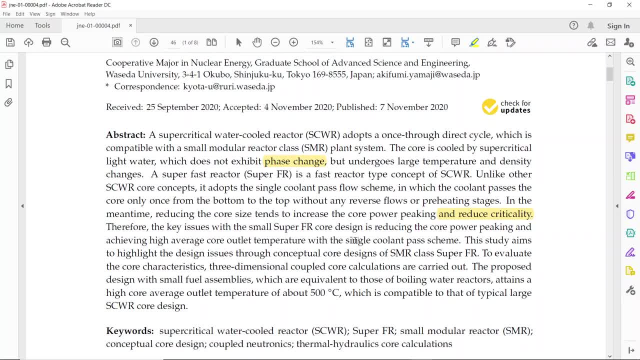 Therefore, the key issues with the small super FR core design is reducing the core power picking. Okay, core power picking, I think it's the variation between the maximum and minimum power within the reactor. So the less homogeneous it is, the more the power distribution, the more the power picking parameter. So it's not good. 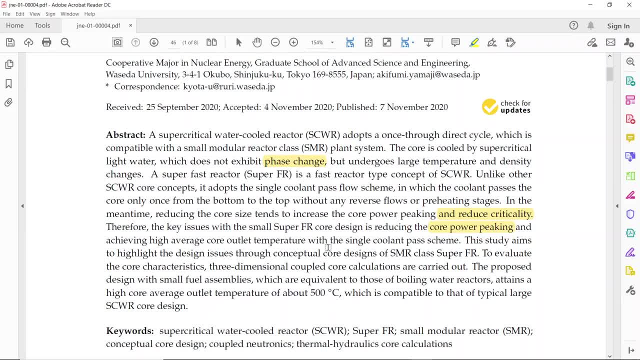 And achieving high average core outlet temperature with the single coolant pass scheme. This study aims to highlight the design issues. through conceptual core designs of SMR class super FR and the three-dimensional couple core calculations are carried out. The proposed design with small fuel assemblies which are equivalent to those of boiling water reactors. 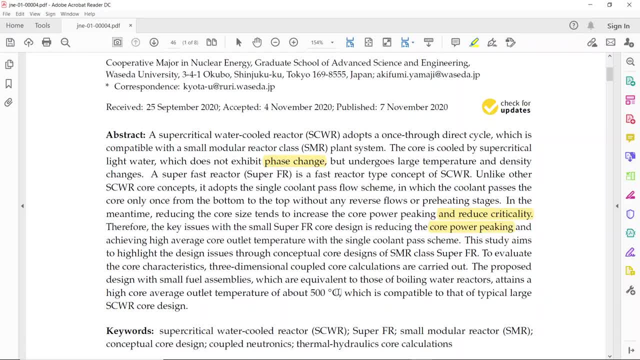 attains a high core average outlet temperature of about 500 degrees, which is compatible to that of a typical large SCWR core design. So you see, the main point of this is to see if we can further reduce the scale of these modular reactors. small modular reactor. 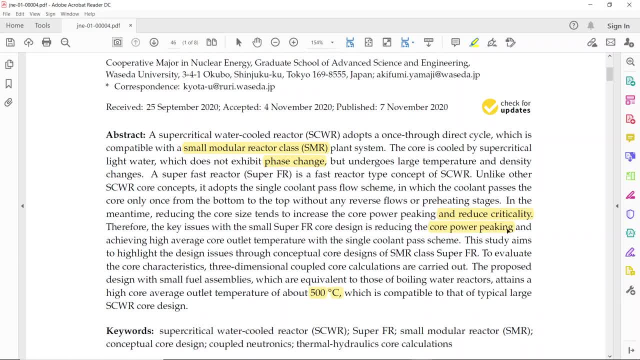 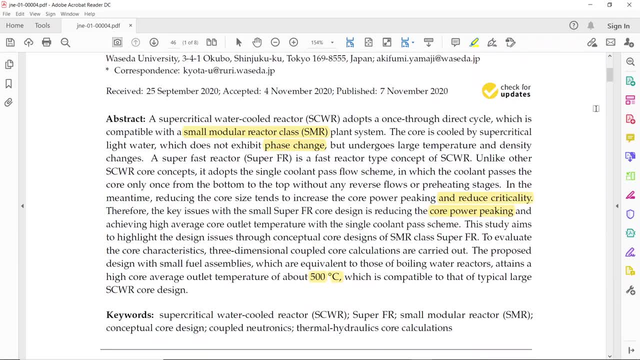 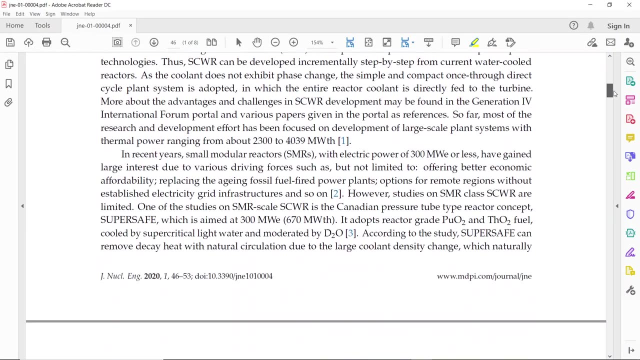 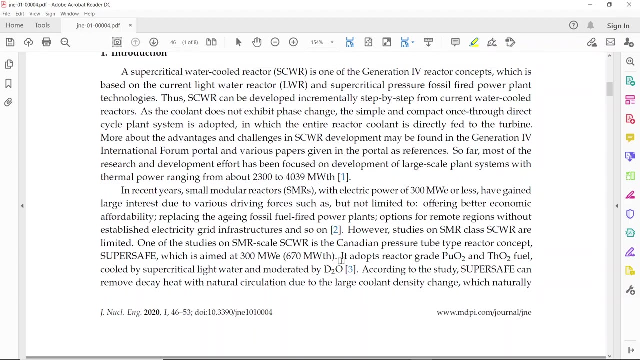 without having the drawbacks of increasing power picking and reduction of average outlet temperature. And for this they use some numerical simulations. but this is a very preliminary stage of the study. It's not yet for design purposes. The introduction it's interesting, but well, yeah, I will mention that. 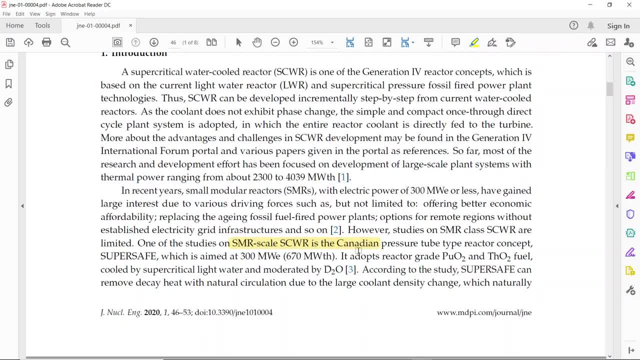 there is this, this Canadian SMR design that uses plutonium dioxide and thorium dioxide as a fuel. That's interesting- Cooled by supercritical light water and moderated by DO2.. I guess DO2 is deuterium water And we will just. 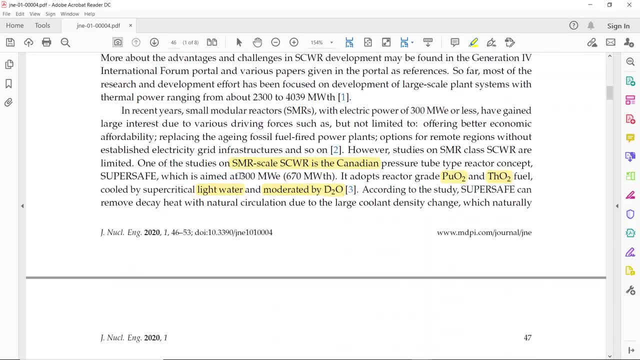 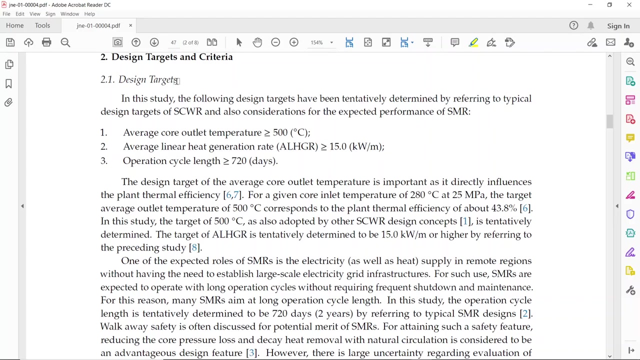 go through all this. Yeah, the power is around 300 megawatts electric, So it's like a bit less than one third of RBMK-1000 or the popular commercial reactors for nuclear production. So we'll jump directly to the design targets. So they fix these targets. So outlet temperature higher than 500 degrees- And this is for thermal cycle efficiency. Below that, you will start losing efficiency. Average linear heat generation rate and operation cycle length. The operation cycle length is the time between fuel recharge. So after this time, which is two years, you need to stop the nuclear reactor. 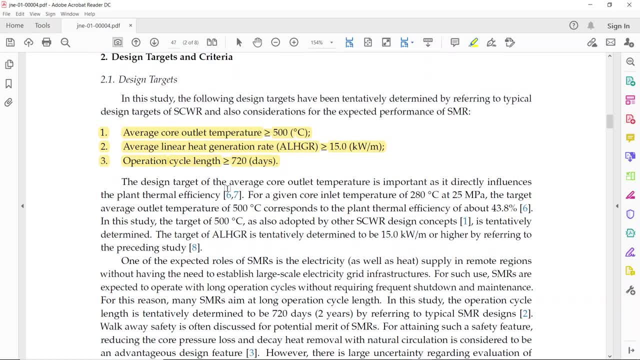 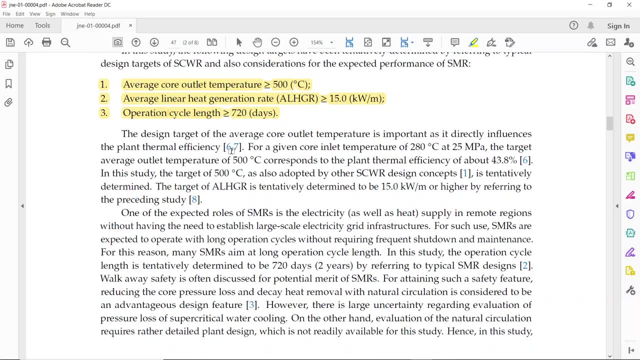 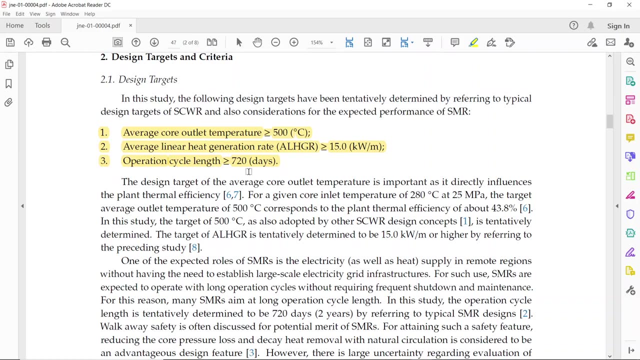 wait for it to cool down and then change fuel assemblies or redistribute them within the core and add some new and then run it again for two years. This is important because in these small nuclear reactors to be cost effective, because they will be deployed in areas very far from 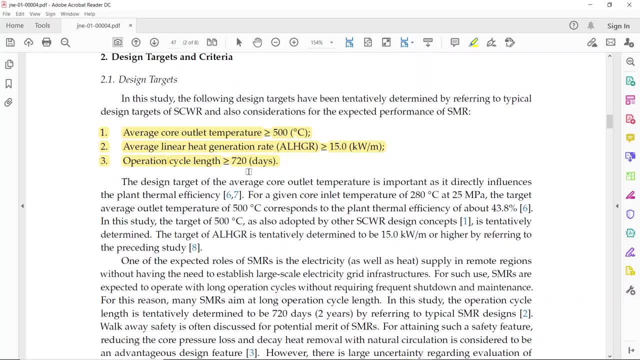 civilization. maybe not civilization, but not I mean. they will be put in Siberia, places which are not very accessible, So having the maximum operation cycle it's critical to for these small modular reactors to be economically viable for the applications they are intended. 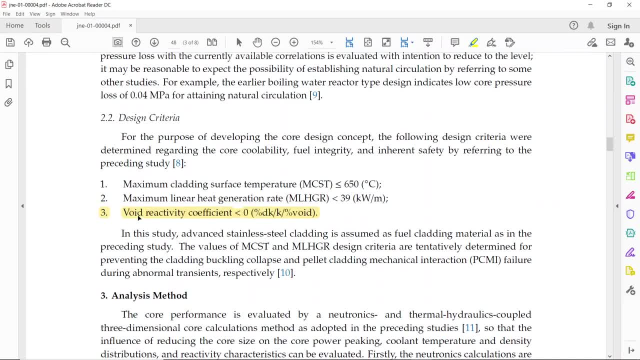 Then we also have this very interesting. One of the certain criteria is the void reactivity coefficient must be below zero. So a positive void coefficient, like the RBMK-1000 reactor, is not acceptable. They impose below zero because these more reactors can only be economically viable if they are inherentlyhow to say this? 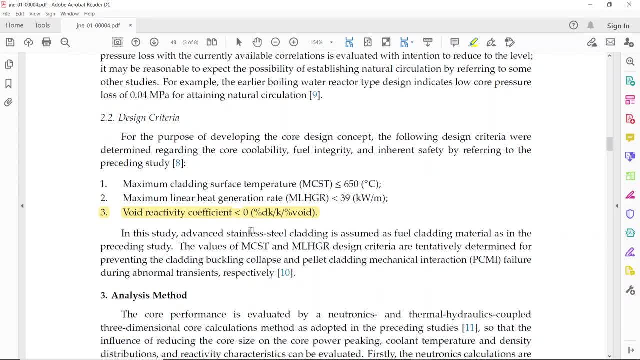 wordby themselves, they are safe. It means when something gets out of hand you just walk aside And thing. they will just stabilize. so for this, of course, you need a negative void coefficient, a positive void coefficient. if you do nothing, it just gets. 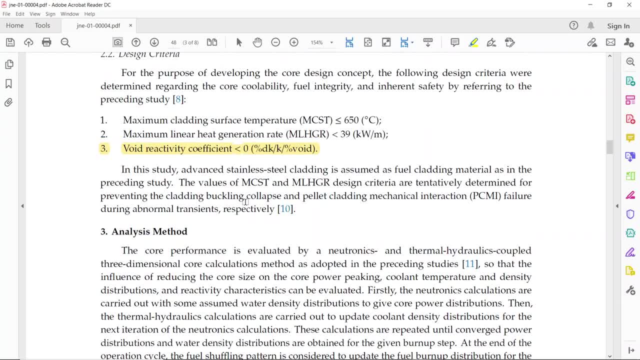 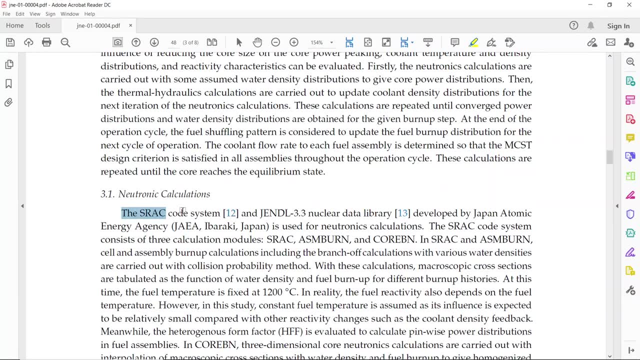 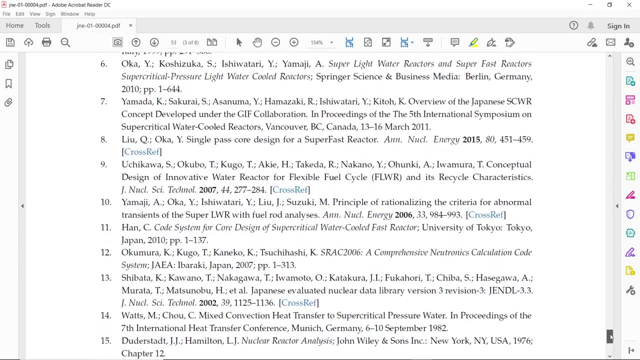 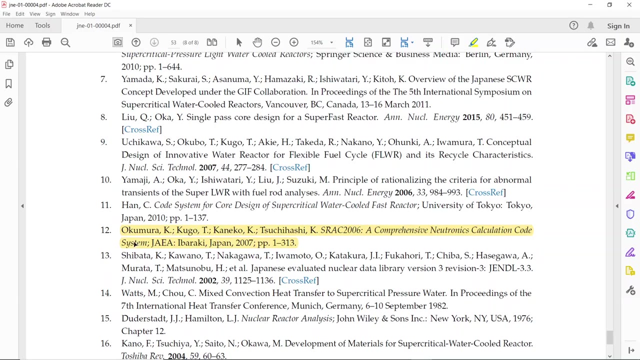 exponential and has a critical runaway and then we get into the model. they use some new sonic calculation that you can check in this reference. I already checked the reference 12. it's a three pages document with a lot of equations in which you have the neutronics and a lot of mathematics associated to nuclear. 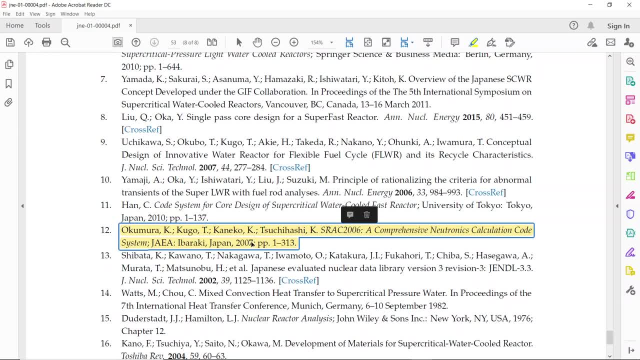 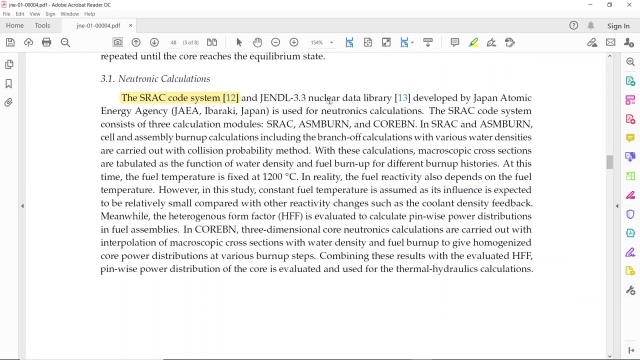 modeling. it seems this 2007, but it must be a. it's based on a previous edition, like from the 80s. the original equations okay, and there are several libraries that you can use for different models for different applications. I will not go deep into this because I don't even 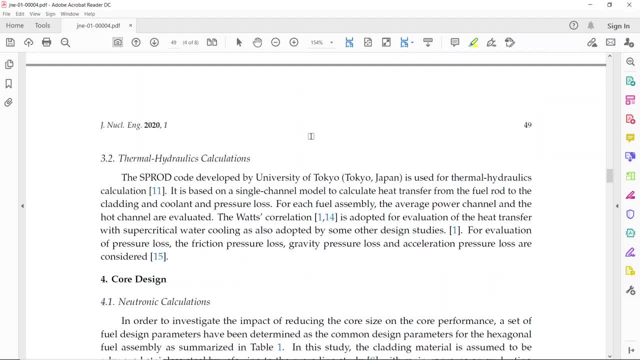 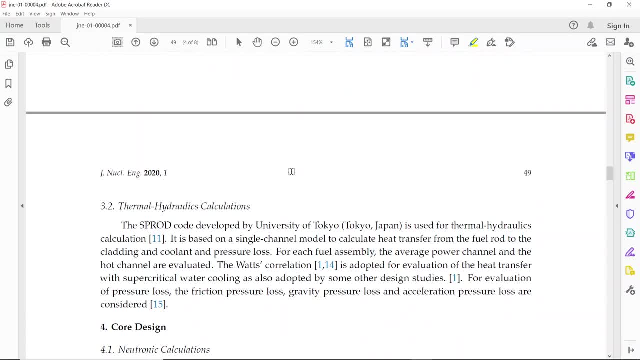 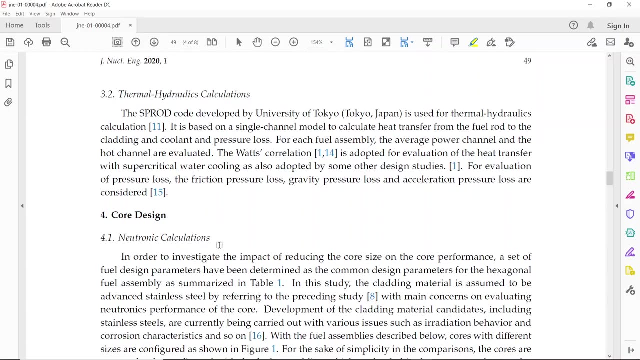 understand everything. so here you have the new neutronics. is this reference we just checked? then we have the thermo hydraulics. so in the model everything must be coupled, because you have the neutronics in the fuel, in the nuclear reaction, and then you have the water that takes out. 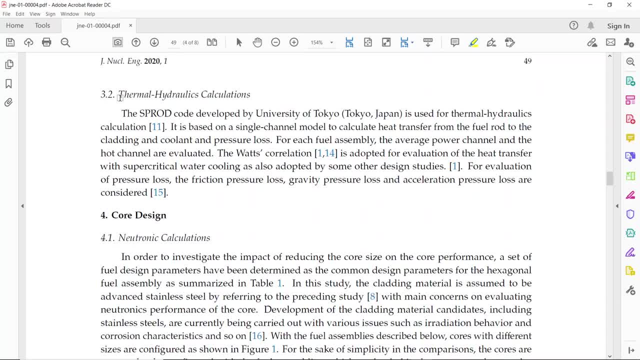 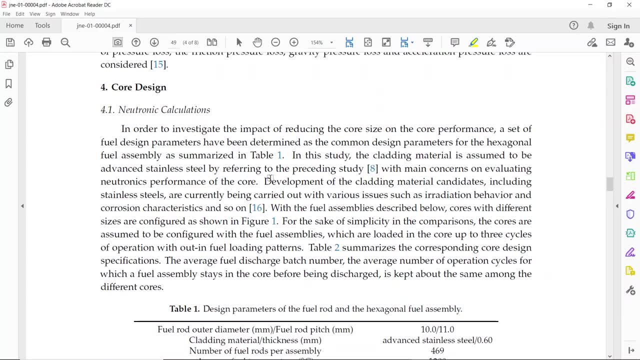 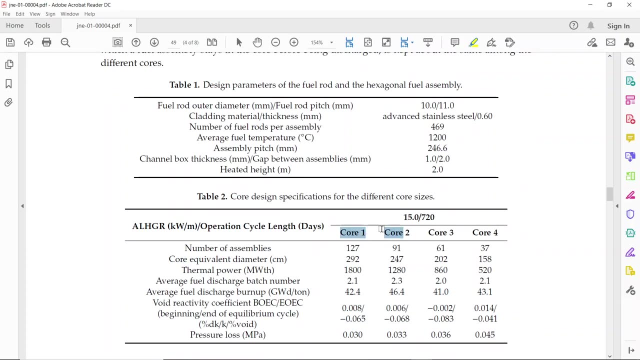 the heat from the fuel pellets and this behaves like a thermohydraulic system. and then we go into the core design and you have all these parameters here. I will not read in detail, but basically they will test 4 core configurations. so each one has a different size, from hundred twenty seven to thirtyset. 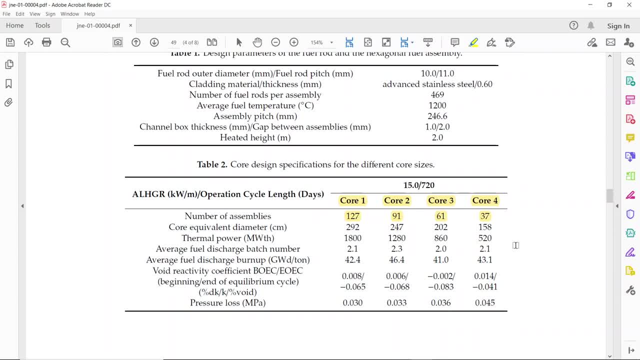 seven foil assemblies. and you are also getting other parameters here, like the average foil discharge batch number, which is in average how many cycles each bundle of foil gets because we reuse- well, we don't. after two years we don't change all the foil assemblies, we change some and we relocate the other. so in average these are the, the, the number of cycles one. 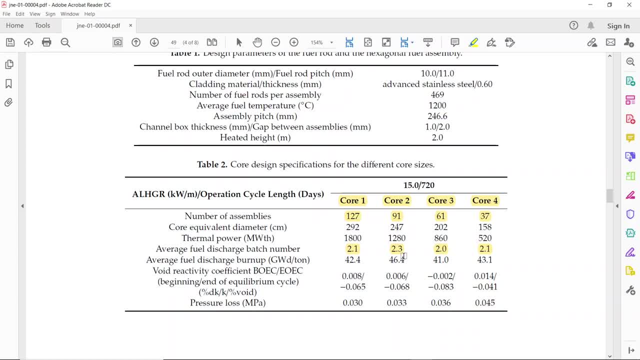 full assembly gets. so the higher the number, the more full efficiency, the more economical you will be. this is also interesting: the average well discharge burn up. so you see, usually with a high average fuel discharge batch number you have, you get a higher burn up so you get more gigawatts. 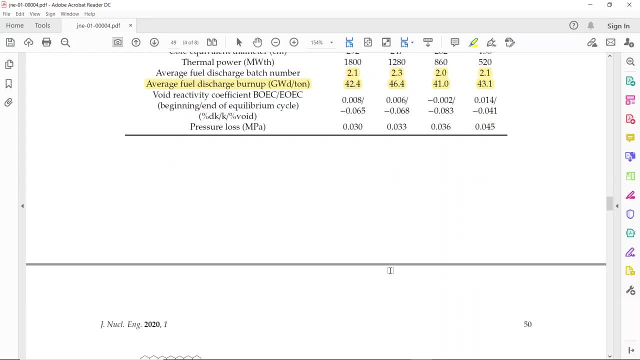 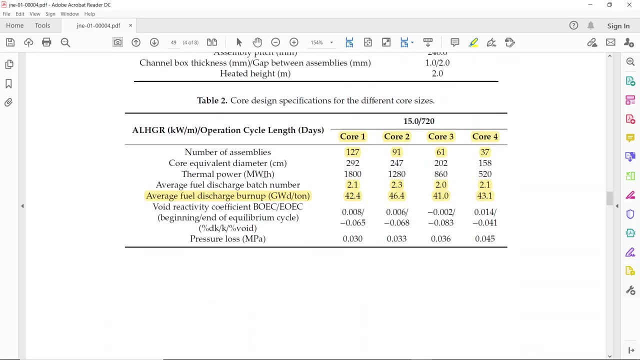 or of the same quantity of foil- and here you see the diagram of the four designs- is the power indicated here, yes, here. so the big is quite big actually. thermal power, this thermal, not electrical thermal, is 1800. the rvmk 1000 is around 3000. so this is almost. 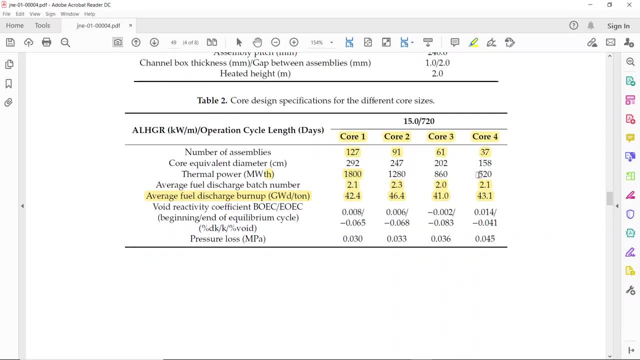 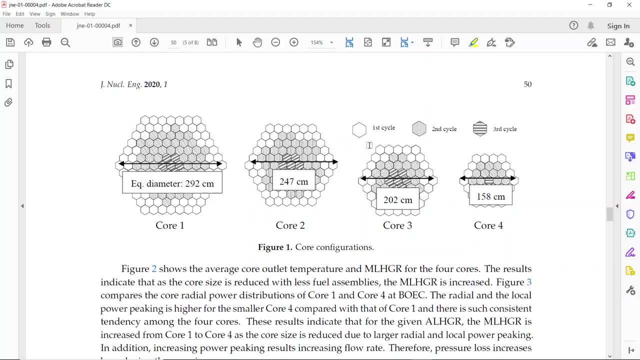 two-thirds of our rvmk 1000 and the smallest is 500, thermal and you see indicated and the fuel cycles. so you put the fresh fuel with more enriched plutonium or or yeah, whatever the foil, you are using uranium thorium, but not all the material is feasible. so 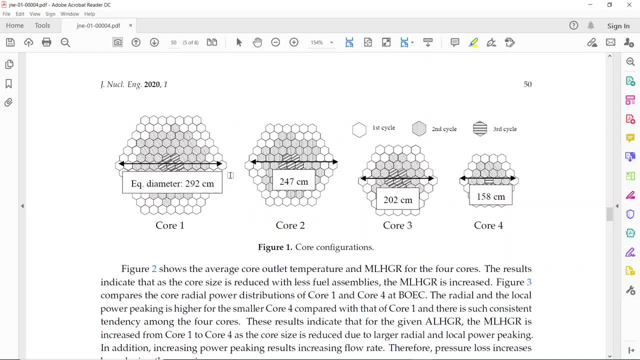 only one part is feasible for, for instance, if you, if you are using uranium dioxide, an enriched fuel element, when it's fresh, before starting the cycle, you are using uranium dioxide, the incredible reason for stopping the cycle will have around four percent of enriched power. incking the cycle will have around four percent of enriched. 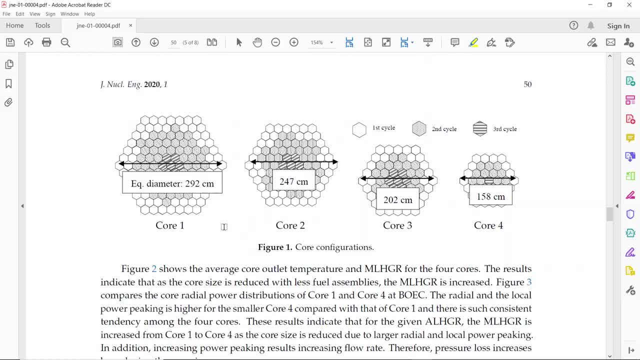 uranium out of all the uranium in the in the assembly. i'm not sure about plutonium, but i guess it's similar and this is called reactor grade nuclear. well, it's very different from weapon grade. for instance, the first weapon that was dropped in the second world war, not the first one that was tested in the desert in the us, the first one that. 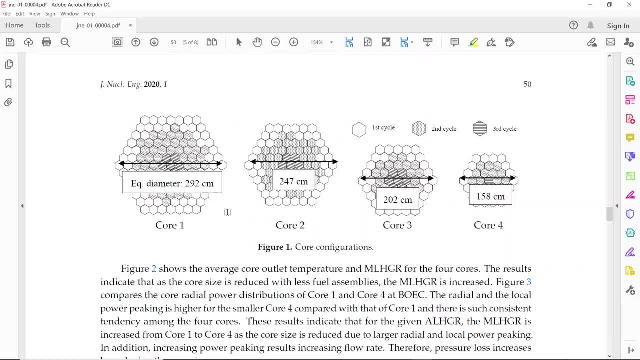 was dropped in japan, which was the little boy was, was a. it was not an implosion bomb, it's the other kind. it's- uh, i don't know how is it called. it's a long, long, thin one. it was called little boy. that one had a uranium core, let's say with a 80 of enrichment. so weapons need a much higher. 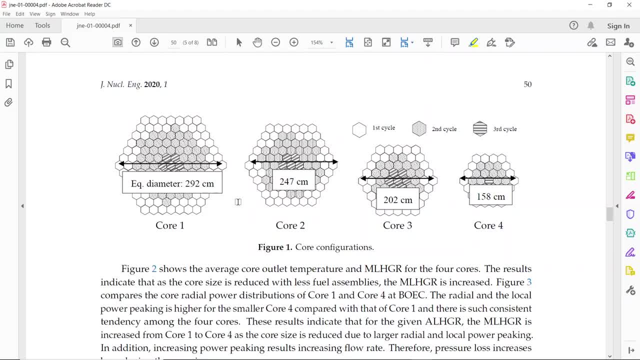 enrichment to be efficient in reactors we have like. we need around four percent in this kind of reactors, in a pressure water reactors, and even no enrichment is needed in can do can do reactors designed in canada or in the original rbmk 1000. before the post accident: 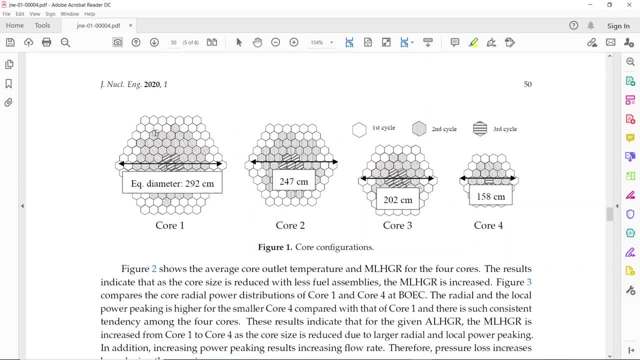 modifications and then as the fuel burned up. burning up, well, not only means that you reduce the feasible material, but also some poison, some poison elements build up in this, in this fuel elements. so the reason why you have this distribution is to avoid power peak, which we saw in the abstract of the paper, so getting the more reactive. well, 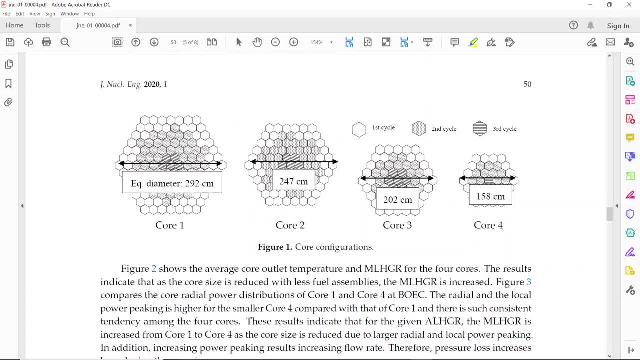 in the middle is the one with three third cycle. so it's it has less feasible and more poison. you get a more homogeneous distribution of power across the reactor and you see here these four configurations and i think this is a flaw of this paper. i will comment on this later, but it's not really a flaw, but maybe a. 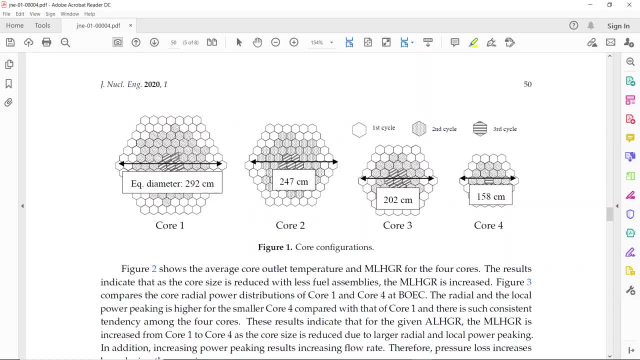 slight weak point because this is very design oriented. you have to choose this configuration. for instance, you cannot here in the center. you need to put seven third cycle assemblies. you cannot put 7.2, which will be the proportional correct value according to the scaling of this problem. 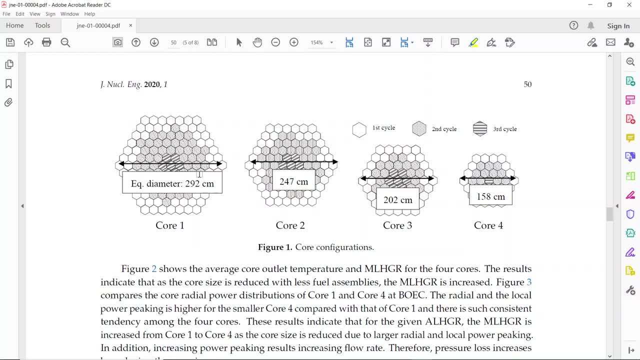 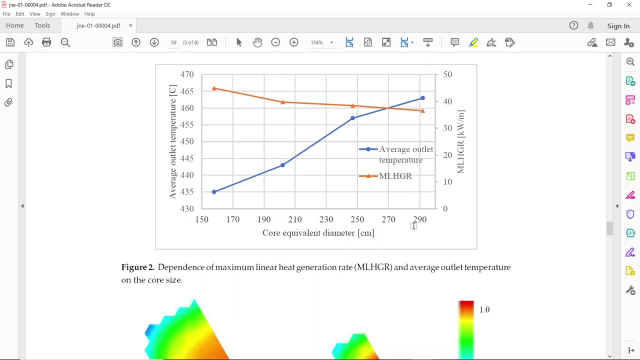 so you are constricted by the discrete nature of this geometry, which makes the next results not very meaningful actually. and here we have the average outlet temperature, which increases with the size of the reactor, which is all the temperature. the higher the better. we have a more efficient thermal system. and here we have some colorful results of the numerical simulation. 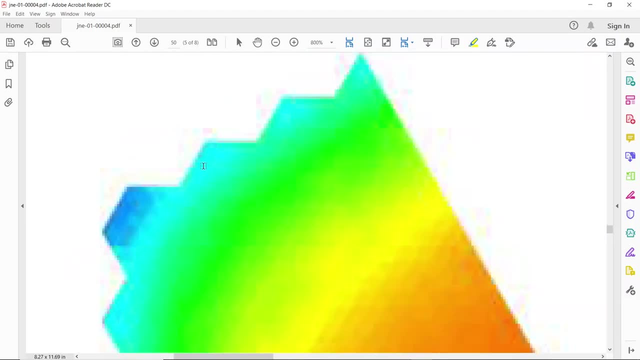 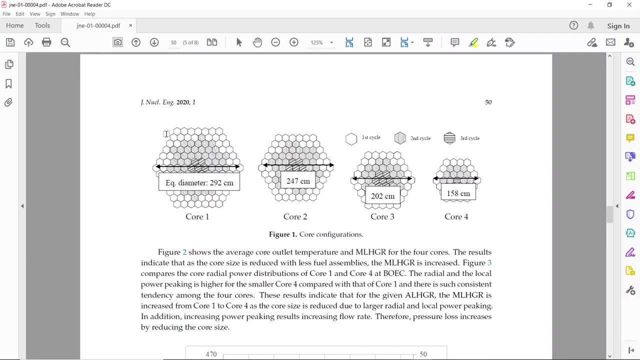 but actually what this picture must be like. one kilobyte, how did they compress this so much? and if you see, the chord has an hexagonal shape, same as vver reactors. this gets a more, a better use of the space than square square shape like the one used in Westinghouse designs. 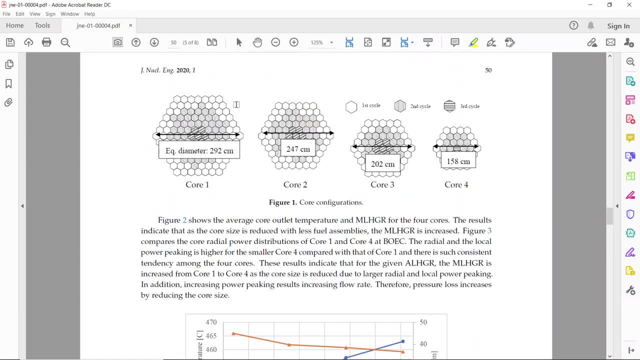 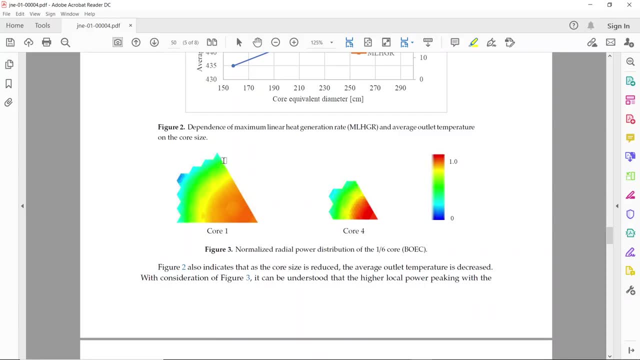 and because of the symmetries. you see this hexagon, so you can cut it like a pizza in six pieces and you have six triangles and they just simulate one, assuming there is symmetry. actually, they could even cut once more, because there is the like, the hexagonal symmetry and then each triangle. 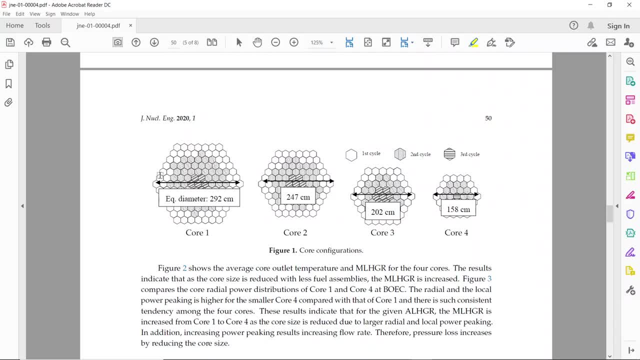 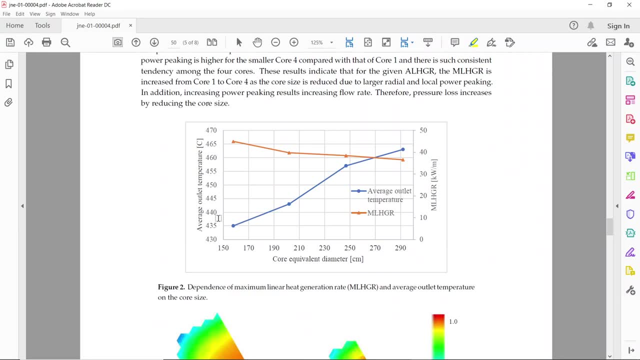 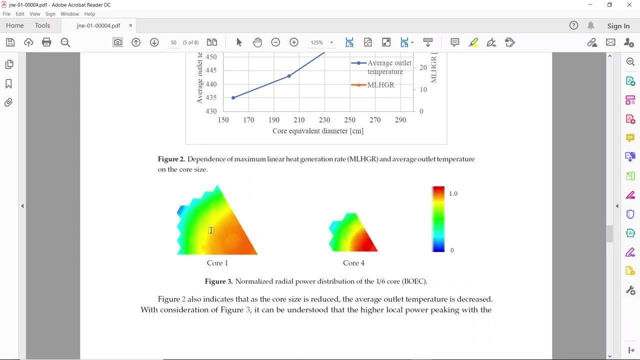 you could still cut it in the middle. it's an isosceles triangle. you cut in the middle, you get two rectangular triangles. so actually you have 12 symmetries here. so if you really wanted to refine a lot this numerical mesh and get a more precise result, you could still cut it into half. why they? 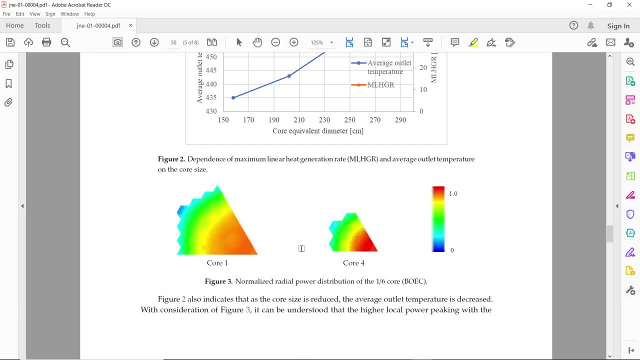 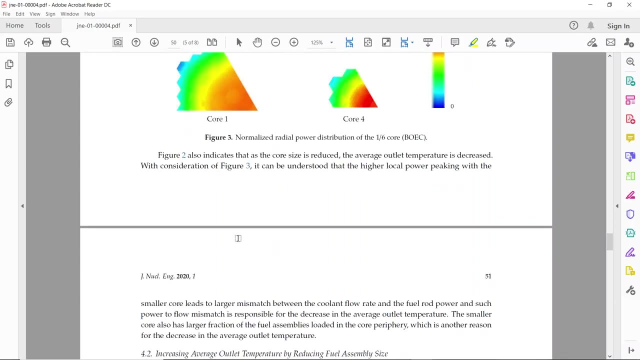 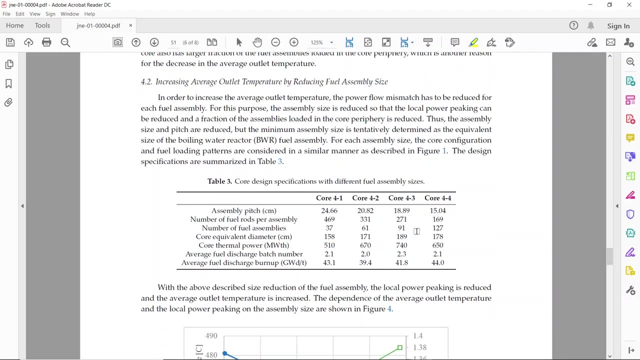 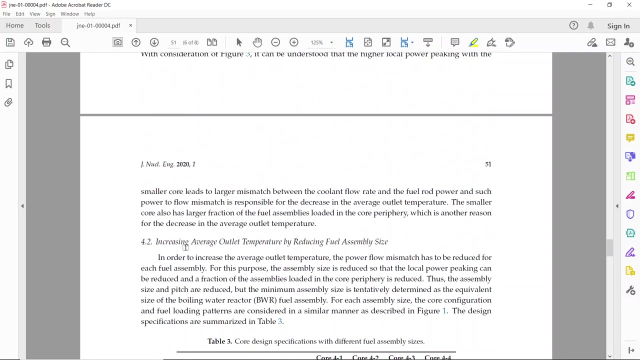 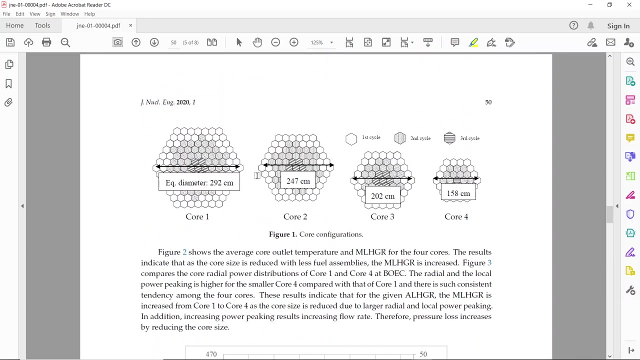 didn't do. i guess it's not really needed because this kind of simulations are not that that heavy. so well, i don't know. and here we have some results. i will not go deep on this, but actually what they propose increasing the average outlet temperature, but yeah, so the conclusion of this is: okay. we have a problem the more we 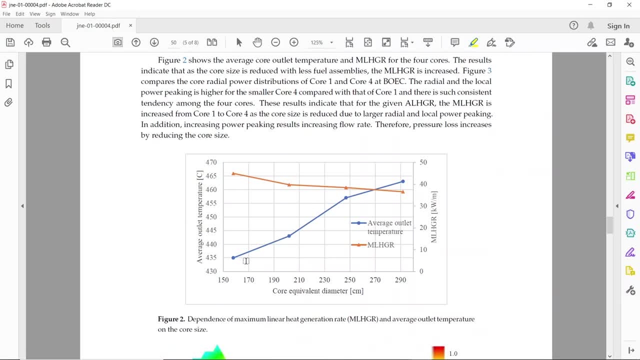 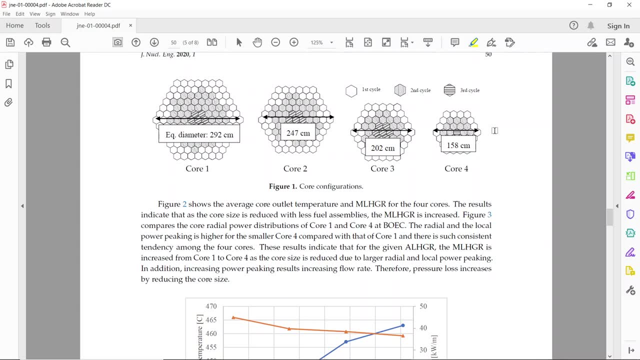 reduce the size of the reactor, the less outlet temperature we have and we have more power peak, which is not good. how to solve this? how can we have small, modular reactors which which are more economically inter, more economically interesting for rural areas, siberia, things like that, or even to put in in vessels to go, these vessels that break? 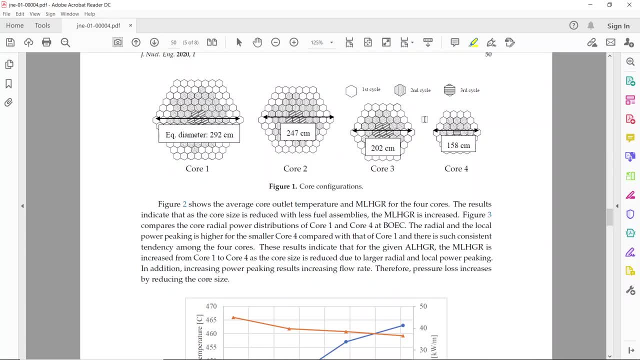 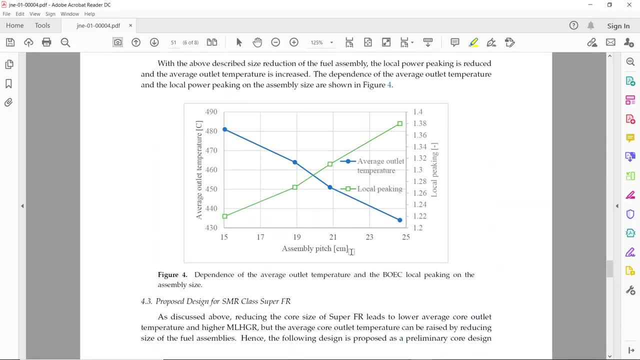 the glass to things like that. so they propose to reduce the size of the fuel assemblies and they do a new simulations and they show that the assembly pitch, which is the size of the foil assembly, the bigger it is, the lower the average outlet temperature and you see it's reducing from 480 degrees to 435 or so. 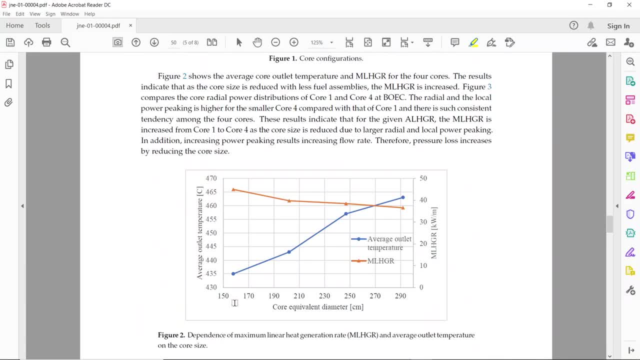 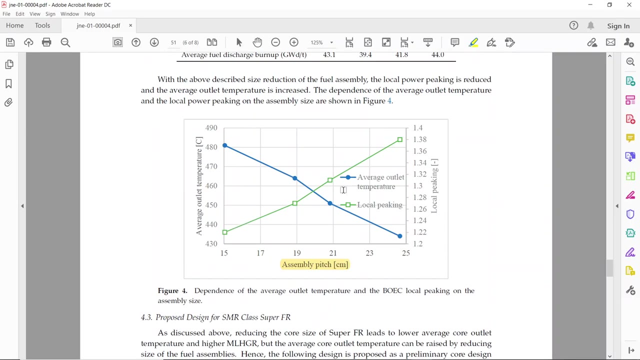 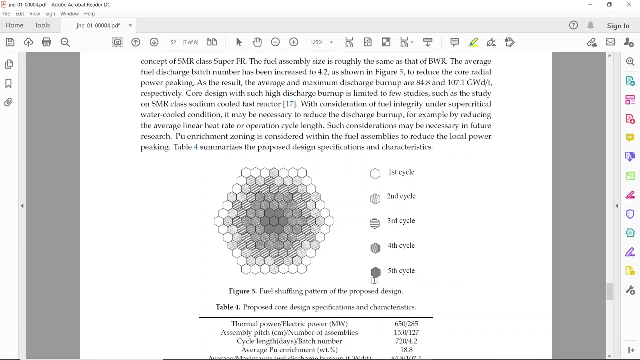 and let's compare this to the previous chart. yeah, so it's in the same scale. so this is very significant, because this reduction of well assembly size compensates for the reduction of size of the actual reactor reactor, assuming that everything else is linear. And then they propose a longer batch cycle. 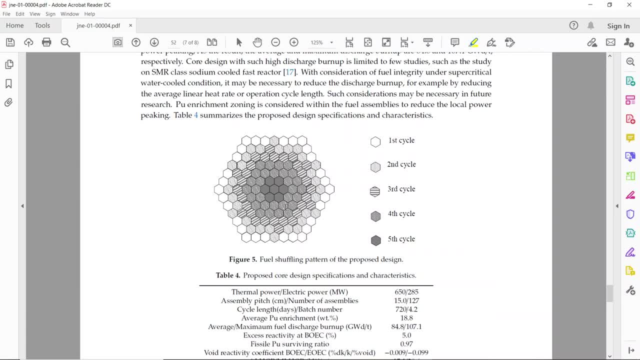 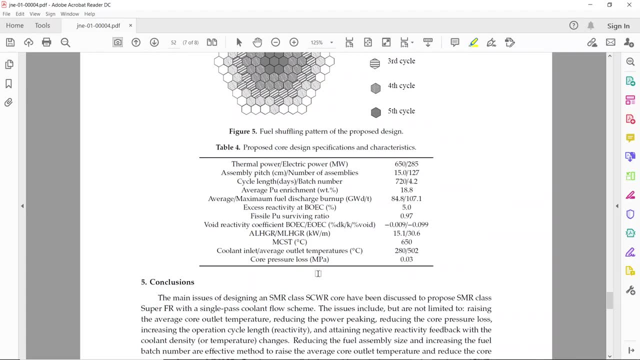 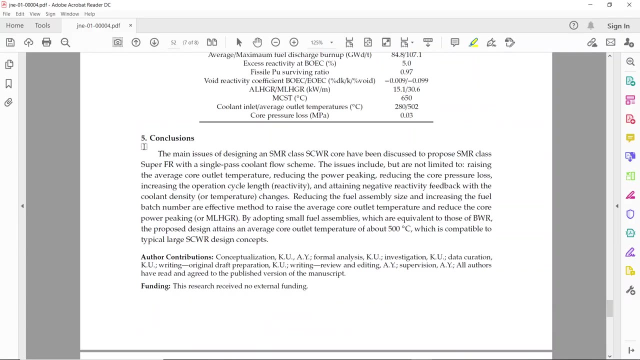 So instead of three cycles they have up to five cycles in the center here, which provides a better use of the fuel. I guess- And I will read the conclusions- The main issues designing an SMR class SCWR core have been discussed. to propose SMR class. 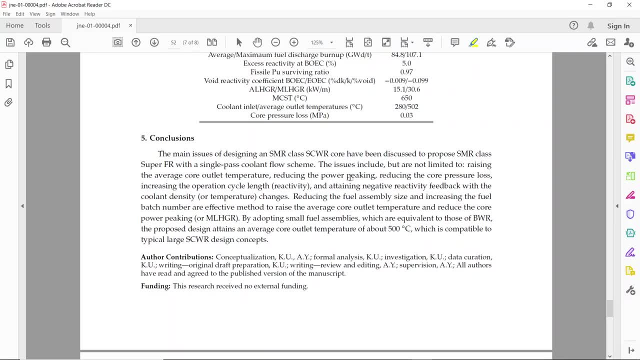 super FR with a single-pass coolant flow scheme. The issues include, but are not limited to, raising the average core outlet temperature, reducing the power peaking, reducing the core pressure loss, increasing the operation cycle length, reactivity- Yes, I don't want to. 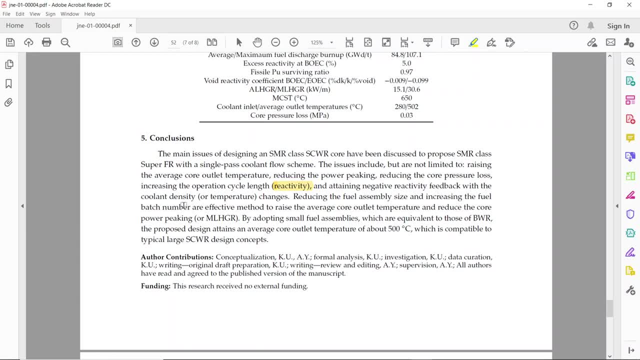 And attaining negative reactivity feedback with the coolant density. This is interesting. also, It's a safety feature, Why it's selecting all the document. Okay Yeah, Reducing the fuel assembly size and increasing the fuel batch number are effective method to raise the average core outlet temperature and reduce the core power peaking. 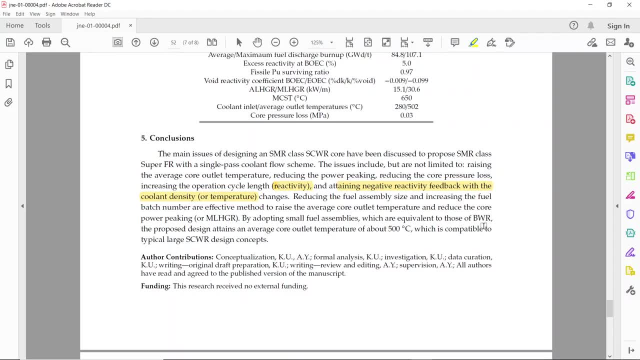 By adopting small fuel assemblies which are- Yes, Yes, Yes, Yes, They're equivalent to those of BW-R. the proposed design attains an average core output temperature of about 500 degrees, which is compatible to typical large SCWR design concepts.